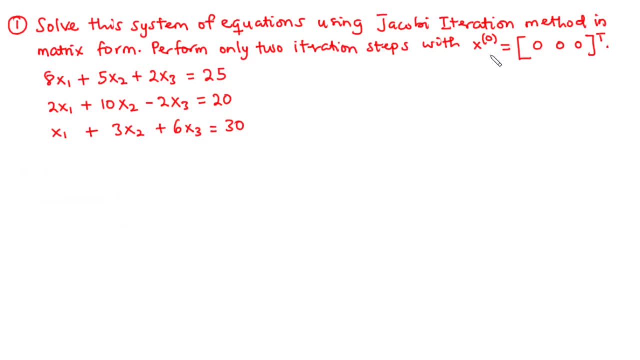 we are asked to perform only two iteration steps, given the initial condition: x of zero equals zero, zero, zero. and then we have this to be the system of equations. So how do we solve this system using Jacobi iteration method in the matrix form? So first of all we need to consider a 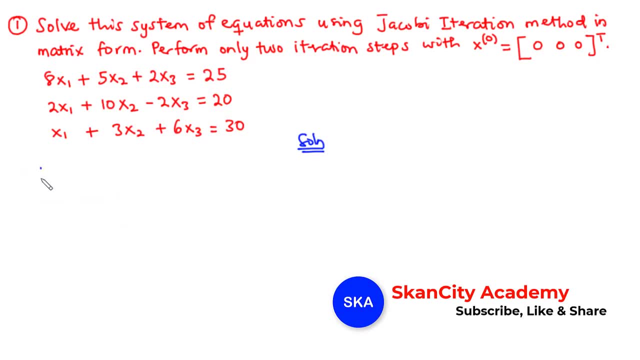 three by three system, which is written in the form: ax equals b. We know a to be the coefficient matrix, x contains the unknown variables x1, x2, x3, and then b represents the coefficient matrix. Now what we need to do here is we need to decompose. we need to decompose the coefficient. 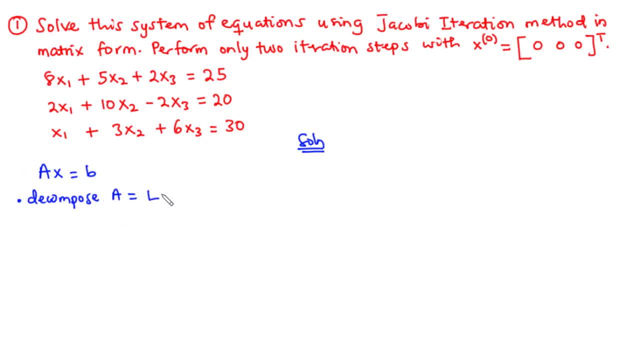 matrix A, so that we have L plus D plus U, Now D. here is a diagonal matrix which contains the diagonal elements of A, And then L is also said to be the lower triangular matrix which contains elements of A strictly below the matrix A. So we need to decompose the diagonal elements of A and then L is also said to be the 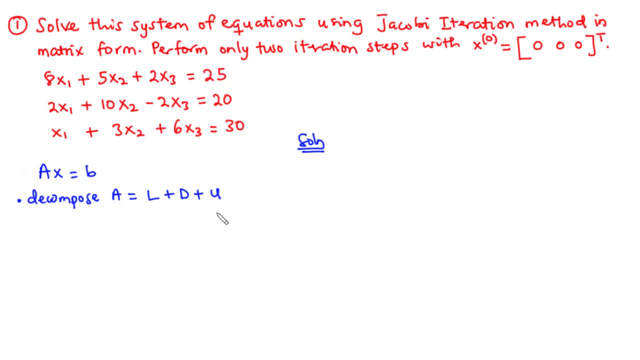 main diagonal, whereas U is an upper triangular matrix which contains elements of A strictly above the main diagonal. Now, putting this expression into this equation- let's call that equation one- putting this expression into equation one in place of A, then we are basically. 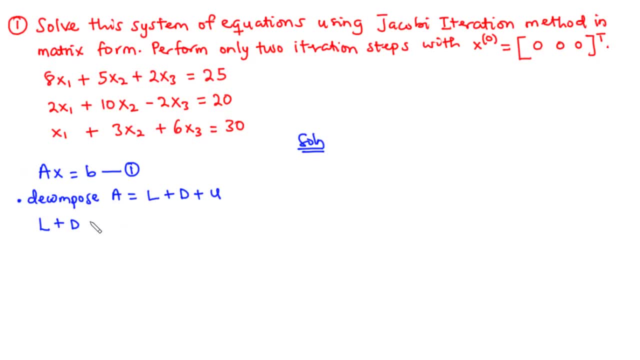 going to have L plus D plus U all times x, and that will be equal to b. Now let's multiply x across, So literally we are going to have L times x plus D times x plus U times x. But then we want to group L and then U on. 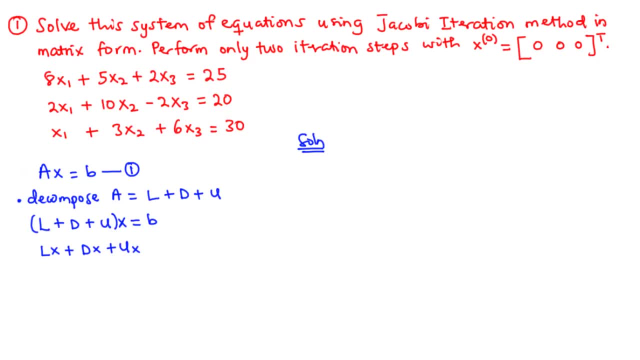 one side, Or basically we want to add L and then U. So what do we do? We multiply x by D, so we have D times x and then plus. we are going to combine L and then U, So we have. 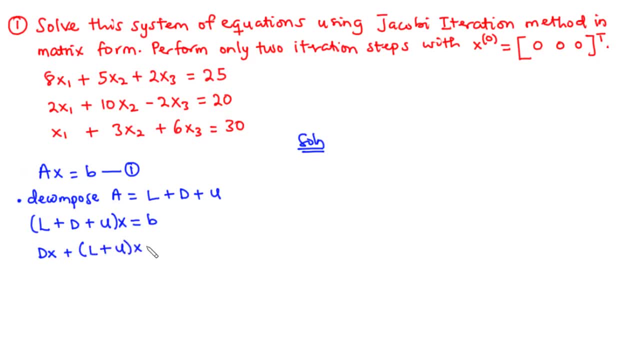 L plus U, all times X. Now, if you expand this expression, you are going to obtain the same expression as expanding what we have here. So we have this: equals equals B. Now, at this point we transpose this part to the right hand side, so that we have dx equals negative. 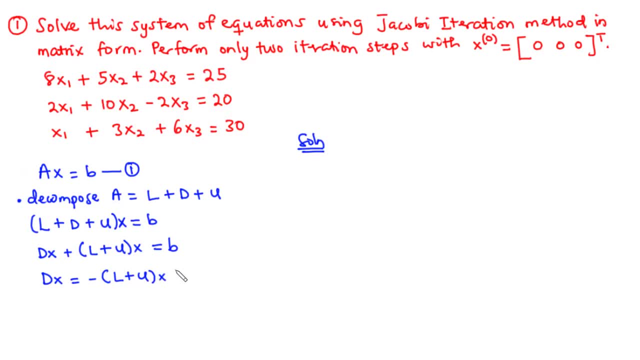 L plus U, all times X plus B. At this point what we want to do is to introduce the X of K and then X of K minus 1 values. So the X of K value is the new value and then the X of K minus 1 becomes the previous or the initial value. So we are going to introduce that in. 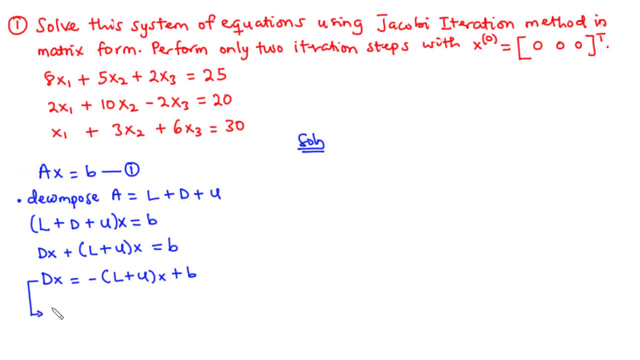 the next step. So we are going to have D times X of K- on the left hand side, That is equal to negative- into bracket L plus U times X of K minus 1 plus B. Now, since we want to find the new value, which is X of K, we divide through by D both sides of the. 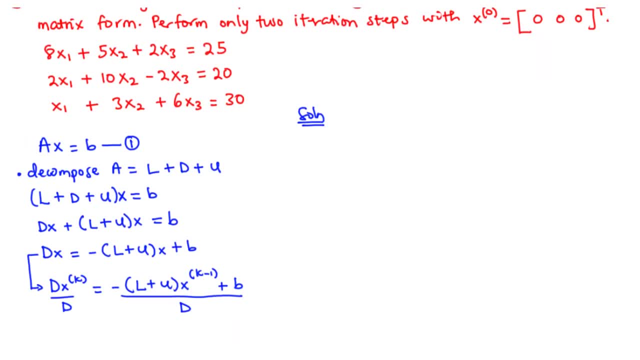 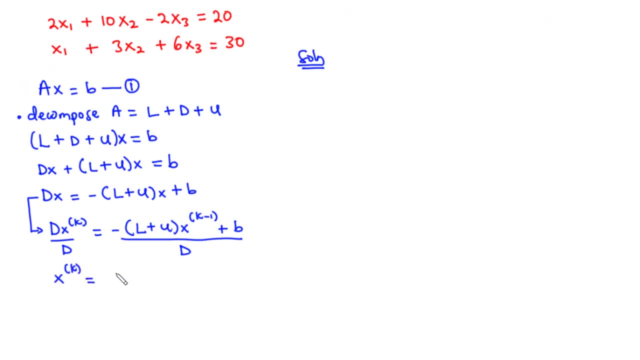 equation by D, So that we have X of K, which is the new value to be equal to. now, because we are dealing with matrices, we have our first part becoming negative D inverse, which becomes negative D inverse Visualization. Okay, so this is negative D inverse And if it is negative, then that is why we have negative. 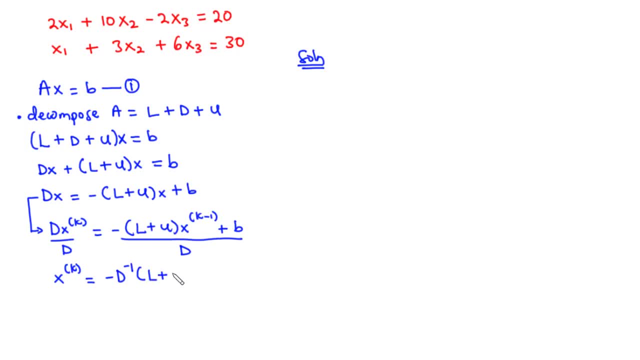 D inverse times into bracket L plus U, all times X to the power of K minus 1, all X, or X of K minus 1 instead of, and then plus D inverse. Now this semblance here is the first part which we see is times b. so basically this is the expression we are going to use to find the new values, or the. 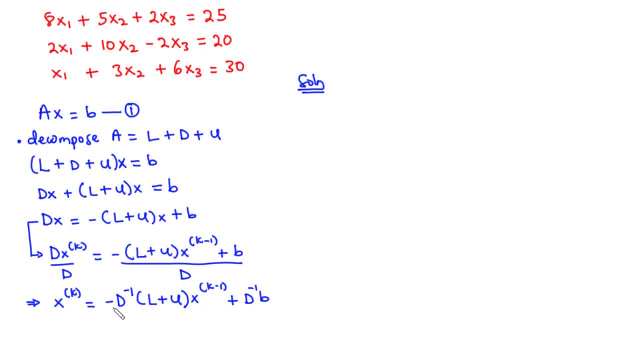 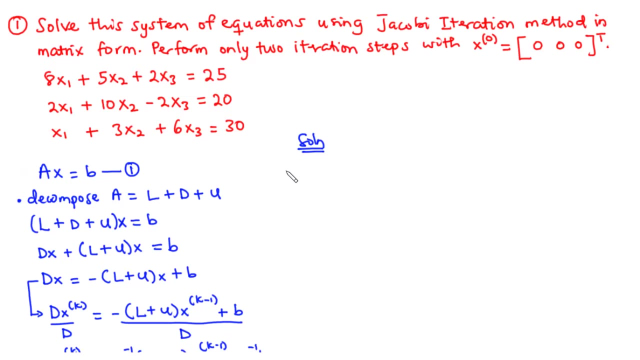 new set of values. now also notice that the expression negative d inverse times into bracket l plus u is said to be the jacobi iterative matrix. now to proceed with our solution. first of all, let's try to pull out the coefficient matrix from this system of equations. so we have 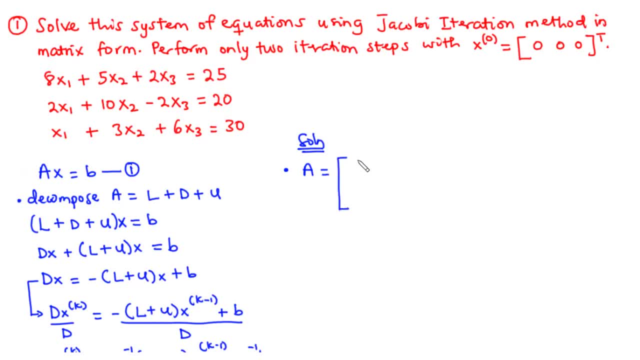 a, the coefficient matrix having elements 8, 5, 2, 2, 10, negative 2, 1, 3, 6, and then we can also have the constant matrix b having elements 25, 20, 20, 30. notice that we have the initial guess to be 0, 0, 0, and then we have this to be our formula. 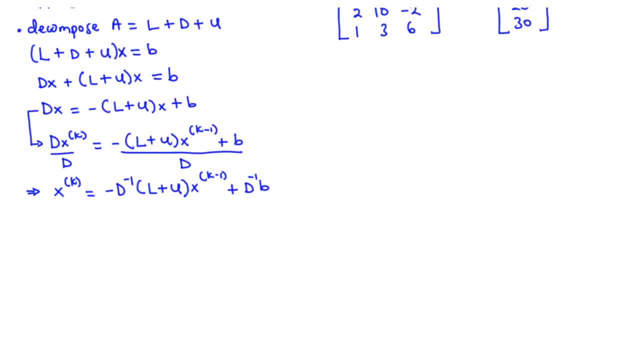 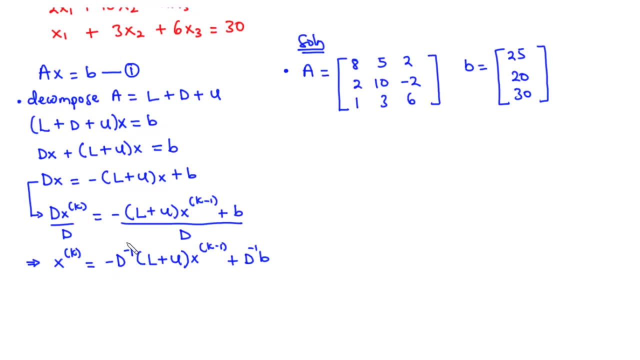 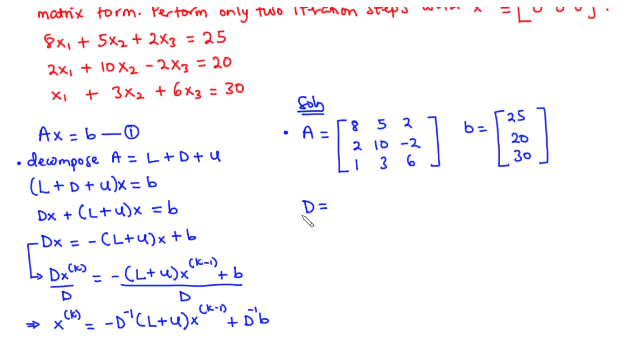 to find the new set of values. so what do we do? considering this formula, let's try to find d so that we can find d inverse. so to find d. d is said to be the diagonal matrix containing the diagonal elements of a. d is the diagonal matrix containing the diagonal elements of a. so what are the diagonal elements? 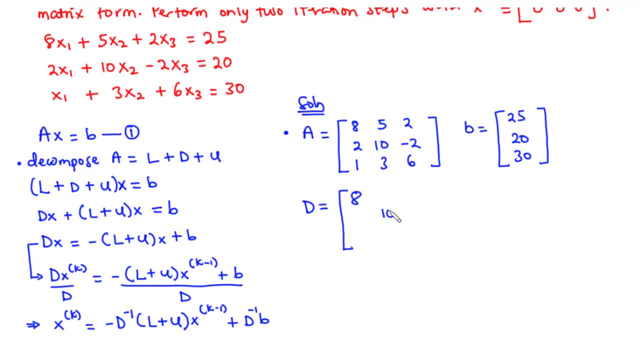 of a, we have 8, 10 and then 6, so the rest of the values are going to be zeros. so this is the matrix d. now, next, we try to find d inverse. so for d inverse, d inverse is basically going to be 0 and the above cut. since d is a decimal, the squares of d are going to be twins, so the 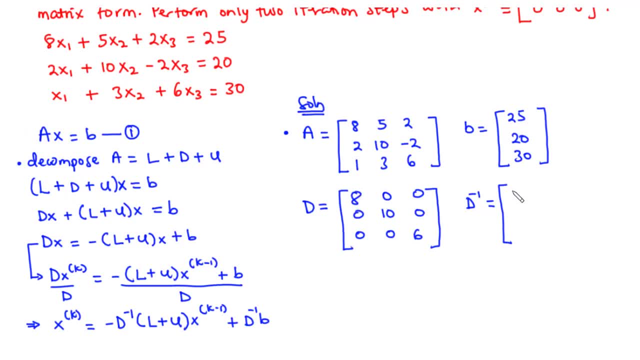 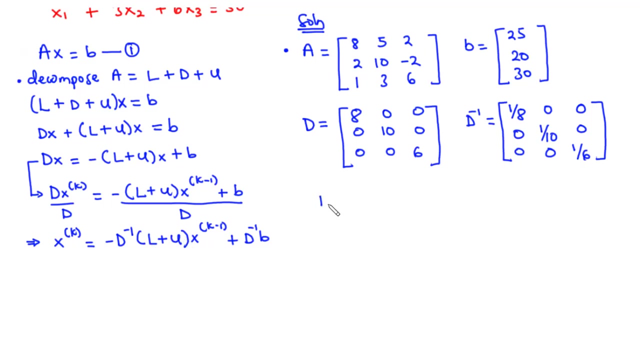 basic ae, зам, ae inverse of d to exist. the main diagonal elements should all be non zeros. if you have even one zero then the inverse of d fails to exist. so we have this matrix to be d inverse, that is, the inverse of d. so after obtaining d inverse, we need to try to combine l and then u now notice that we have l. 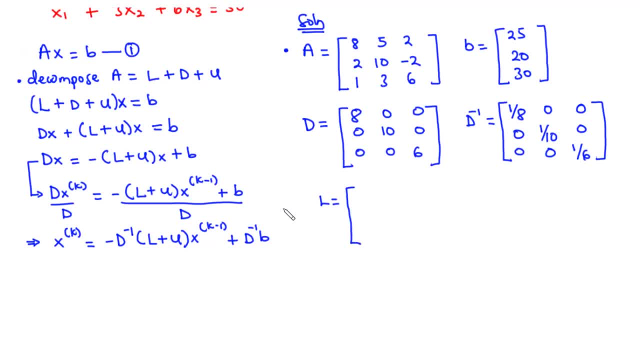 to be the lower triangular matrix which contains element of a strictly below the main diagonal. so we have this to be a element of a below the main diagonal or strictly below the main diagonal are two, one and then three. so we have two, one, three. the rest of the values are going to be zeros. 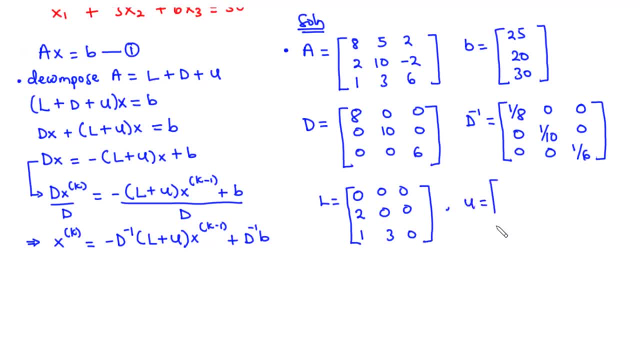 similarly for u, that is the upper triangular matrix containing all elements strictly above the main diagonal. so we have zero, zero, zero, zero, zero, zero. and then we have five, two negative two. so this is l and then u respectively. so to find l plus u, we are basically going to add corresponding 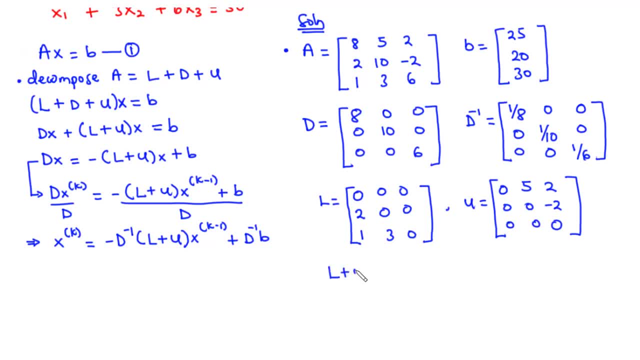 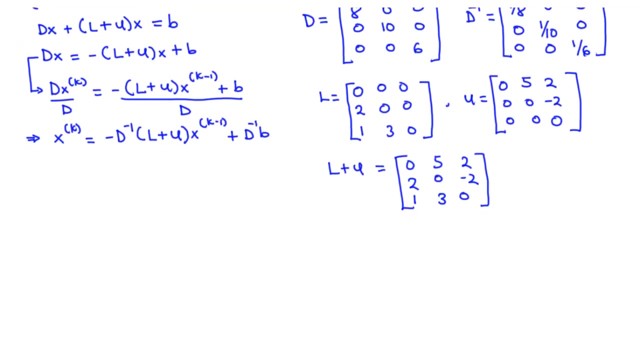 components or elements. so we have l plus u and that is giving us. we are going to have main diagonal elements or zeros. and then we have five, two negative, two, two, one, three. so this is l plus u. so at this point we can have the jacobi iterative matrix, which is given by negative. 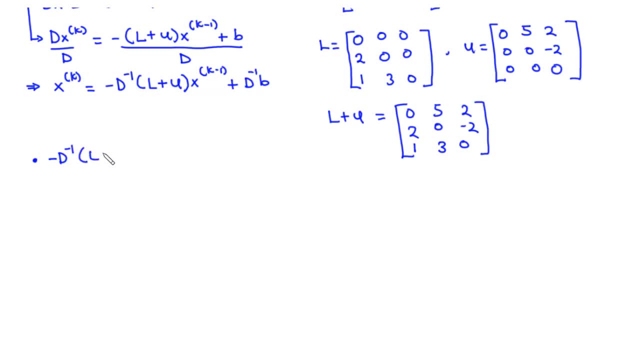 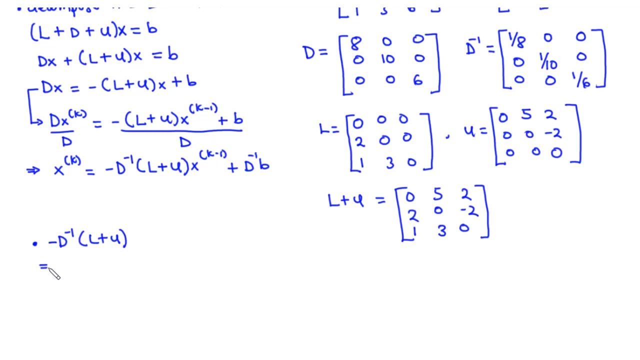 d inverse into bracket L plus U to be equal to. we have D inverse, we have D inverse to be this metric. So we can have this here: 1 over 8, 0, 0, 0, 1 over 10, 0, 0, 0, 1 over 6.. 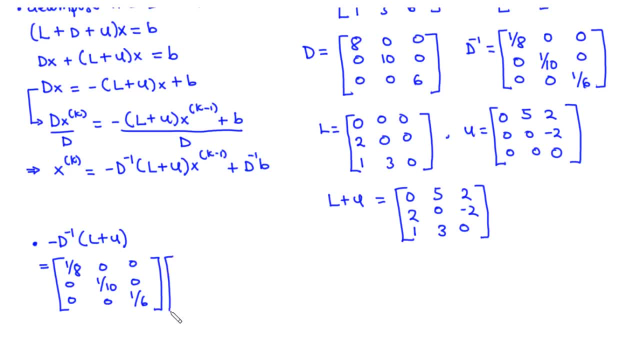 Times L plus U. this is the combination. so 0, 5, 2, 2, 0, negative 2, 1, 3, 0.. Let's try to multiply these two matrices, So we have a 3 by 3 matrix, multiplying another 3 by 3 matrix. 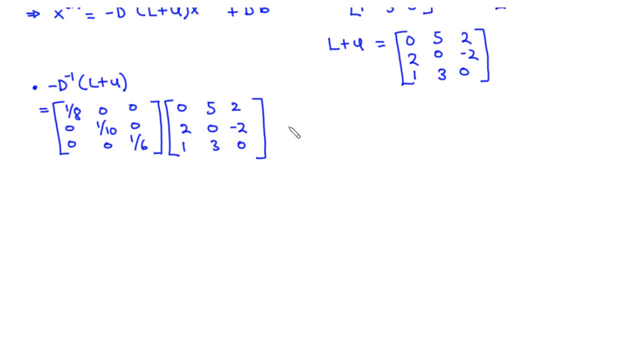 We are going to obtain another 3 by 3 matrix, So the resulting matrix is going to be 3 by 3.. Notice that this is negative D inverse. So we are going to have a negative here. We are going to have a negative here. 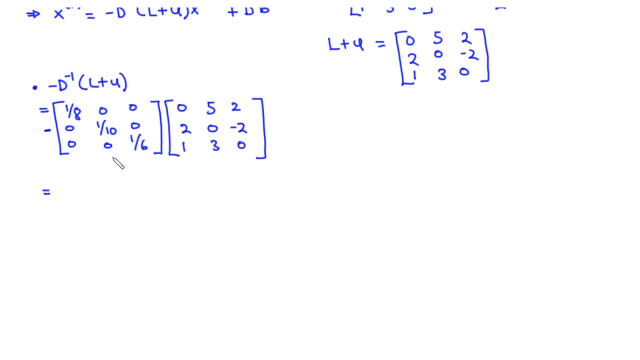 Notice that this is a diagonal matrix, So we can have a shortcut in multiplying these two matrices. But if you want to use the traditional approach, you can multiply first row, first column, first row, second column, first row, third column, to complete one row. 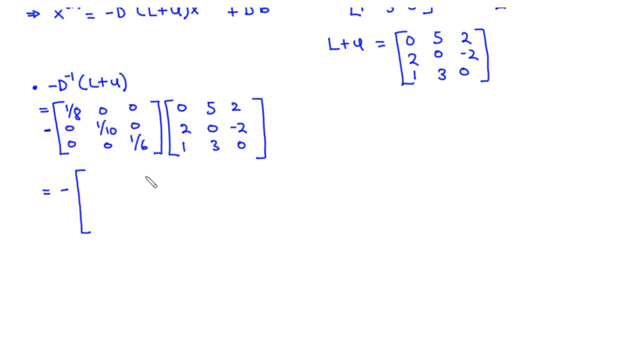 And then you do that for row 2.. And then you do that for row 3.. But then, in order to use the shortcut, we basically make sure that all the diagonal elements are 0. And then, next, we multiply this value by these two values to complete the first row. 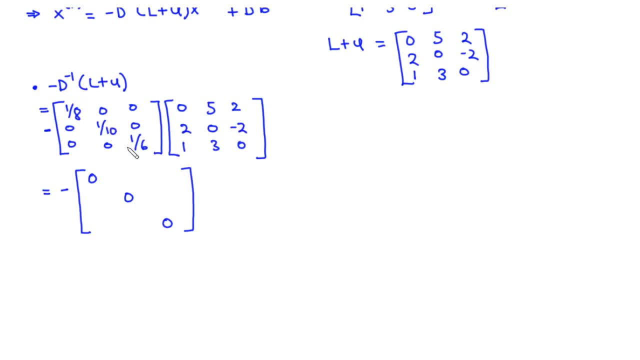 We do this for these two values to complete the second row, and then that's for the third row. So we are going to have 1 over 8 times 5, which is simply 5 over 8, 1 over 8 times 2, that becomes 2 over 8.. 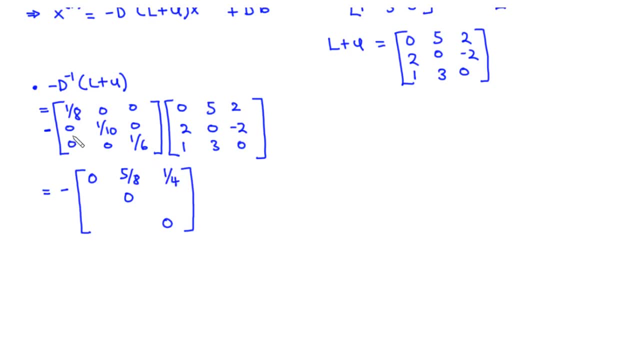 We cancel out, then we have 1 over 4.. We are going to have 1 over 10 times 2, that is 2 over 10, so that becomes 1 over 5.. And the same thing happens here. 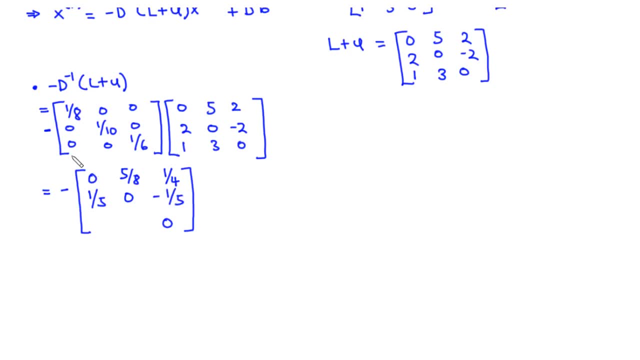 Just that we have a negative, So negative 1 over 5.. For the last row we have 1 over 6 and then 3 over 6, which is 1 over 2. And then we multiply negative across. 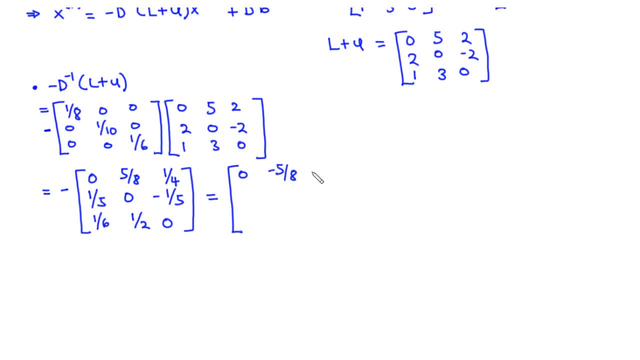 We have 0, negative 5 over 8, negative 1 over 5.. Negative 1 over 5.. Negative 1 over 5.. 4. next row, we have negative 1 over 5. 0 1 over 5, because there is a negative here and then last. 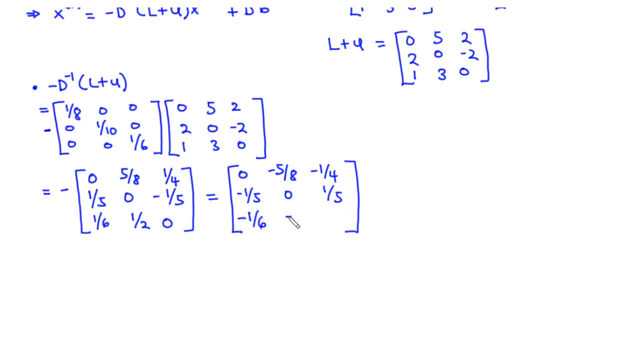 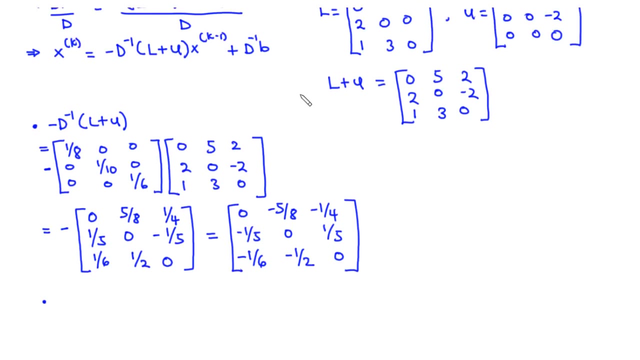 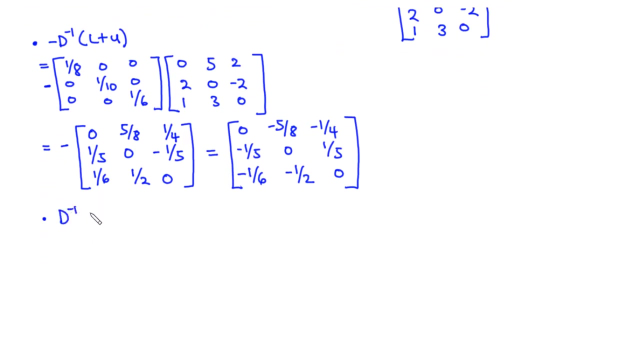 row, we have negative 1 over 6 and then negative 1 over 2, 0. so this is the resulting matrix for this expression, that is the Jacobi iterative matrix. now let's move on to the second part of the equation, that is D inverse times B, the inverse times B. so we have D inverse to be 1. 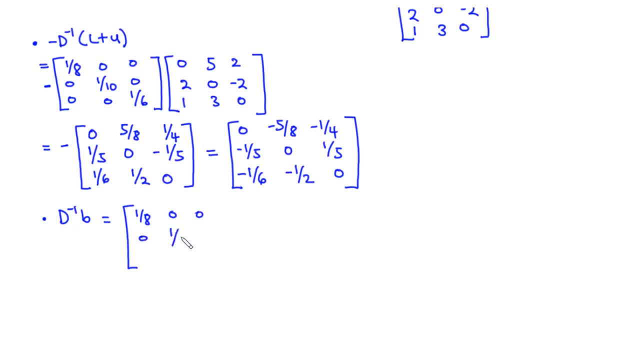 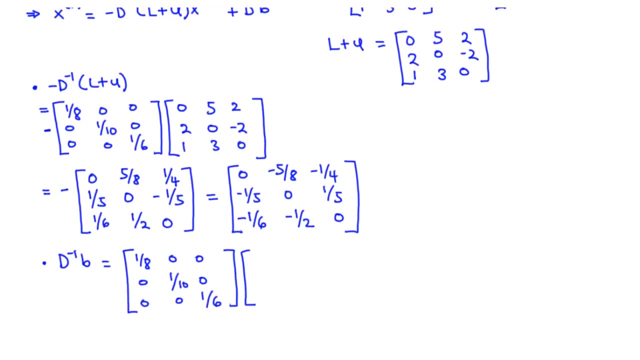 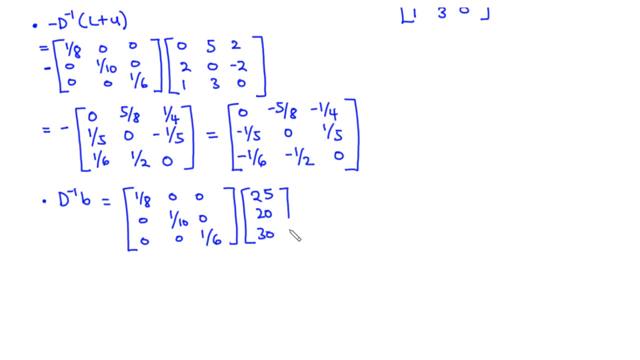 over 8 0 0 0, 1 over 10 0 0 0, 1 over 6 times the constant matrix B having components 25, 20, 30, so 25 20, 30. so let's try to multiply these two matrices. we have a 3 by 3 matrix. 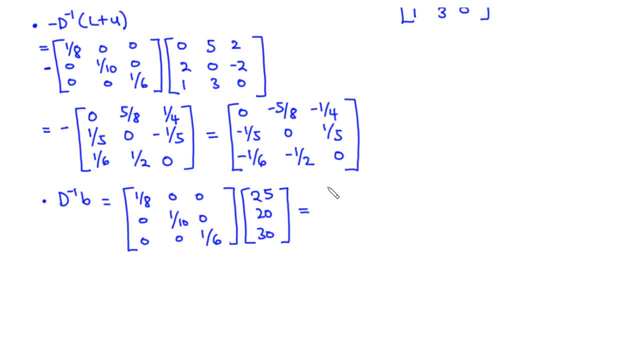 multiplying a 3 by 1 matrix. so the resulting matrix is going to be a 3 by 1 matrix. so the clue is: we multiply this by that, this by that and then this by that. so 1 over 8 times 25, we have 25 over 8. 1 over 10 times 20 is 20 over 10, which is 2, 1 over 6 times 30, that's. 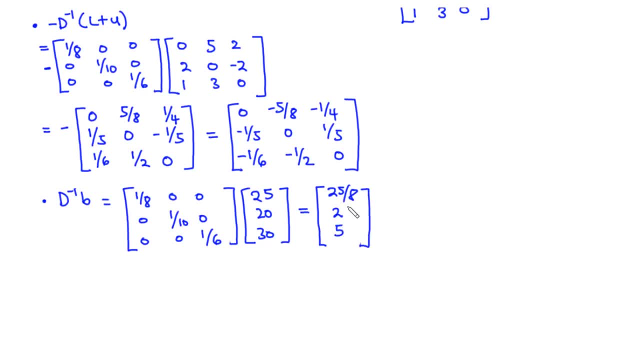 going to be 5. so this is the result or the resultant matrix from this expression. so, considering the formula to find the new set of values x of k, we are going to have x of k to be equal to x of k of negative 3 times the subtracting 1 over 4. so let's check this out as well. 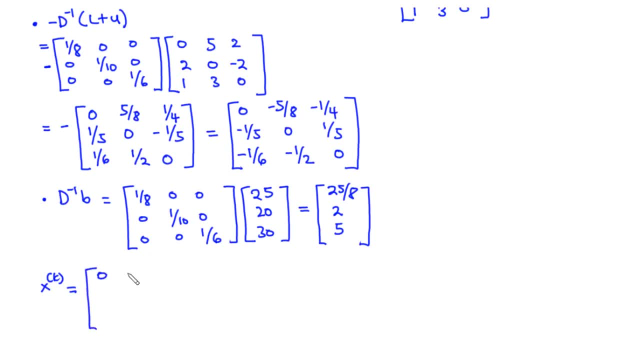 so for this expression, this matrix expression or this matrix that is, 0 negative, 5 over 8 negative, 1 over 4 negative, 1 over 50, 1 over 5 negative, 1 over 6 negative, 1 over 2, 0 times. 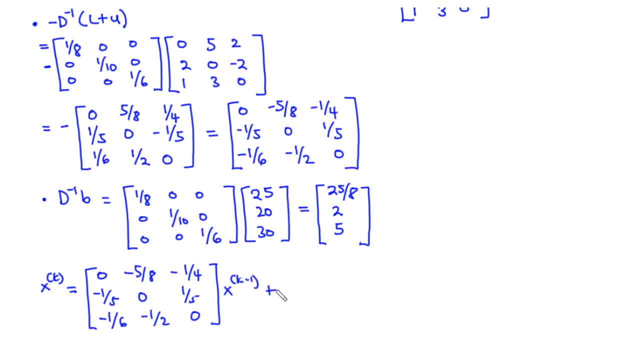 x of k minus 1 and then plus 25 over 8,, 2, 5.. So, basically, this is the formula we are going to use to find the new set of values. So let's consider the first iteration step. 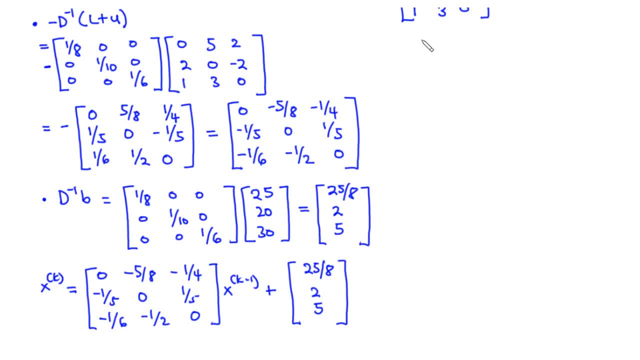 Let's consider the first iteration step. So for the first iteration step, first iteration, we have k to be equal to 1.. So we find k of 1.. Sorry, k of 1. And that is going to be. 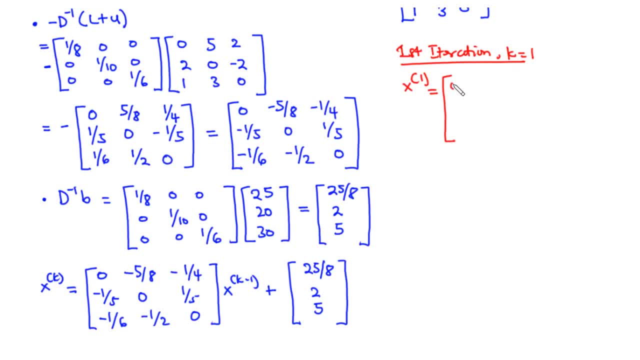 we have this matrix: 0, negative 5 over 8, negative 1 over 4, negative 1 over 5, 0, 1 over 5, negative 1 over 6, negative 1 over 2,. 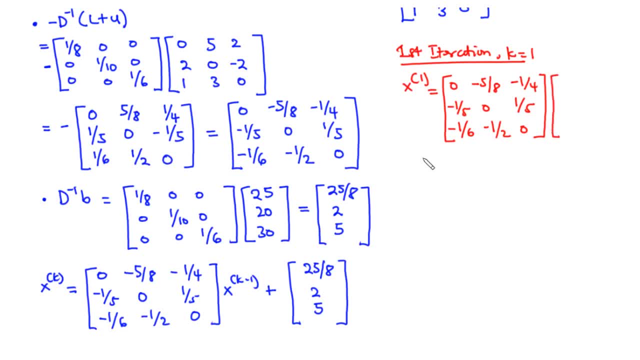 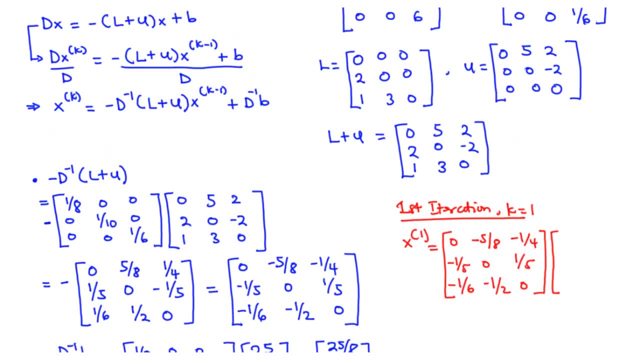 0 times here becomes x of 1 minus 1, which is x of 0.. Now we have x of 0 having components 0, 0, 0. So this becomes 0, 0, 0,. 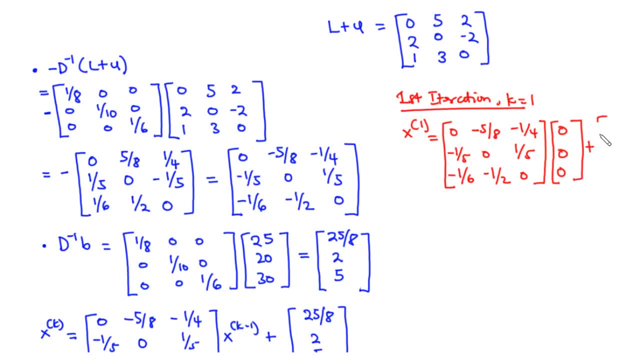 plus the matrix having components 25, over 8,, 2, and then 5, 5.. Now notice that we have this to be a color matrix, having all its components to be 0. So it means that when you multiply this matrix by that, 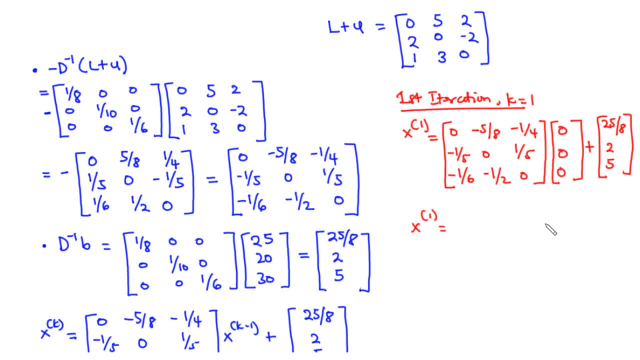 you are going to have all 0's. all the entries are going to be 0's. So 0, 0 plus 25 over 8, that becomes 25 over 8, 0 plus 2 is 2,. 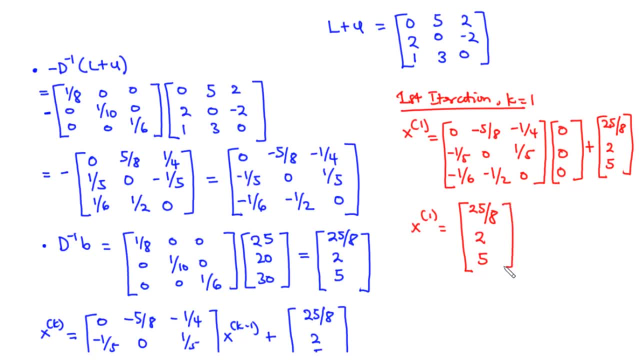 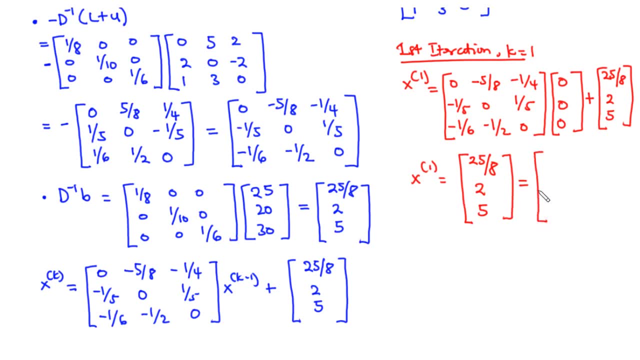 and then 0 plus 5. is also 5.. Now we can represent this as this mouse in 6 significant figures, so that we have 3.12500, 2.000, 00 and then 5.000, 00.. So this is. 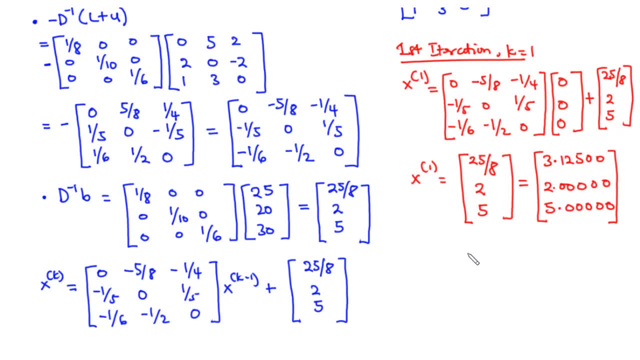 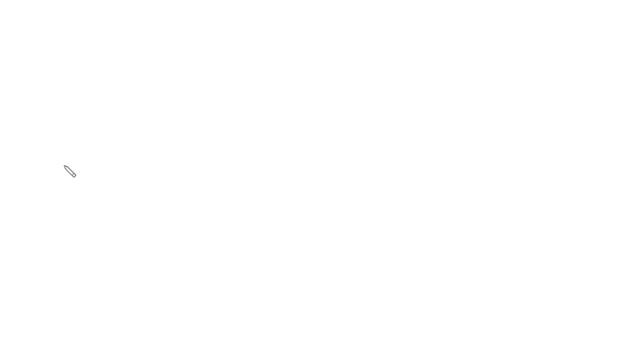 the set of values that we obtain after the first iteration step. So let's do the second iteration step. So for the second iteration step, we are going to have k to be equal to 2.. Therefore, we have x to be equal to 2.. So we already obtained the matrix equation. so we have this to have. 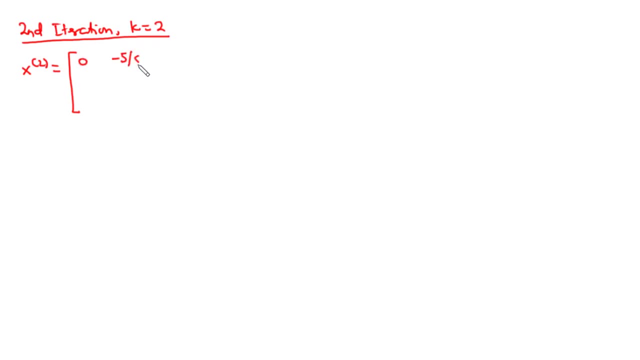 components: 0, negative 5 over 8, negative 1 over 4, negative 1 over 5, 0, 1 over 5, negative 1 over 6, negative 1 over 2 and then 0 multiplying. So this time we are going to have: 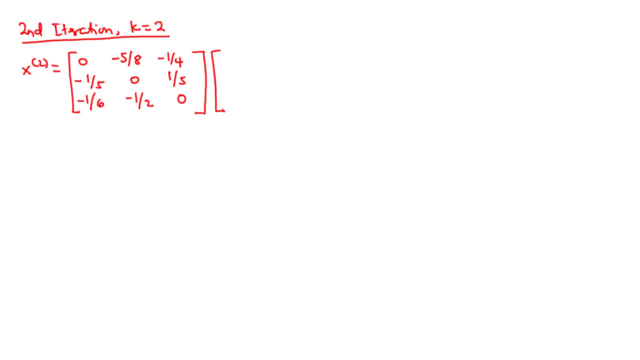 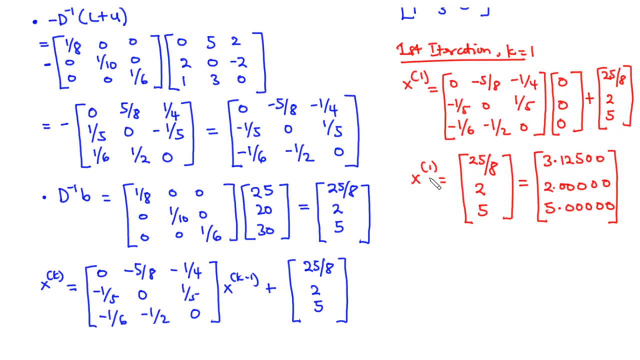 x of 2 minus 1.. We are going to have x of 2 minus 1, which is x of 1.. Now the set of values of x of 1 are the values that we obtained here, So 25 over 8,, 2 and then. 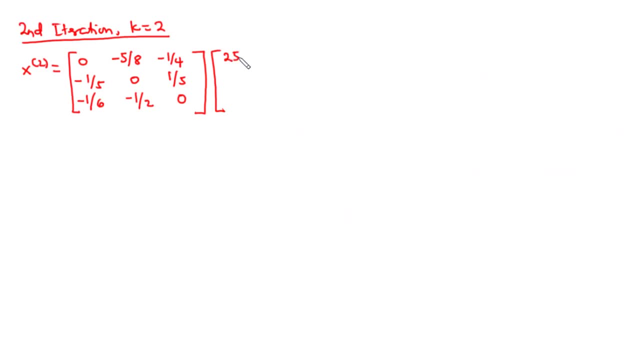 5.. So 25 over 8, 2 and then 5.. And then we have this plus, according to the formula plus 25 over 8, 2 and then 5.. So let's do the calculation. So we are going to multiply this matrix. 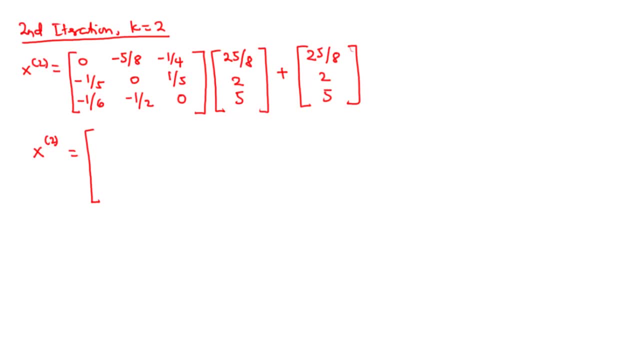 by that matrix. This is a 3 by 3 matrix. We multiply that by a 3 by 1 matrix and we are going to obtain a 3 by 1 matrix. So we multiply row by column, Row by column, So 0 times. 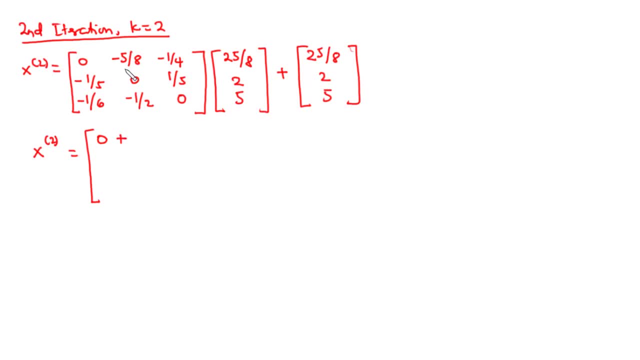 25 over 8, that is 0 plus negative 5 over 8 times 2. That becomes negative 10 over 8 and that becomes negative 5 over 4.. So negative 5 over 4 plus negative 1 over 4 times 5.. So that: 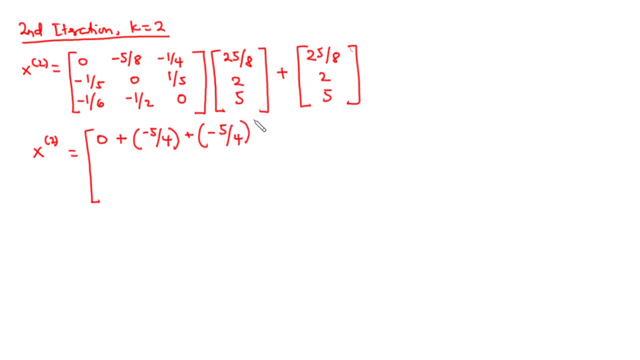 becomes negative: 5 over 4.. And then here we are going to have 25 over 8,, 2, 5.. Now for row 2, we have negative 1 over 5 times 25 over 8.. So 5 goes here. 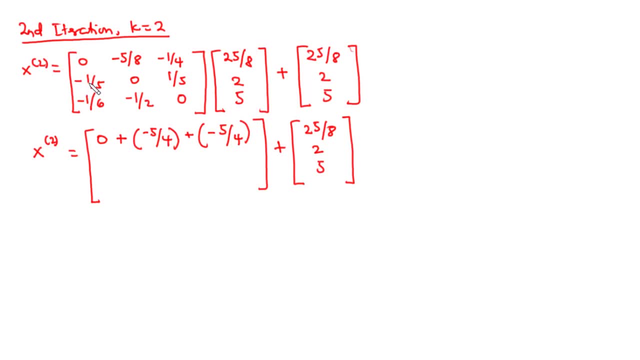 once 5 goes here 5 times, That becomes negative 1 times 5.. So negative 5 over 8.. 0 times 2 is 0. And then we have 1 over 5 times 5, that is. 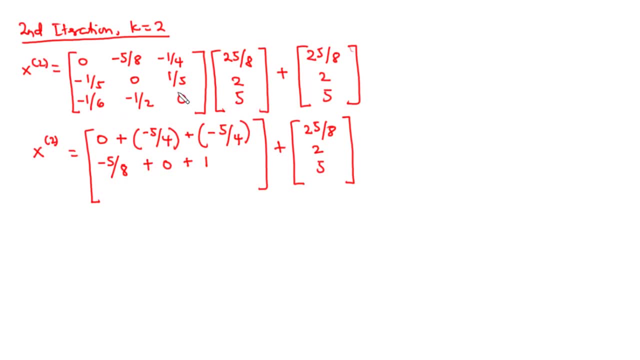 1. For the last row, we have negative 1 over 6 times 25 over 8.. Negative 1 times 25,. that is negative 25.. 6 times 8, 48.. Negative 1 over 2. 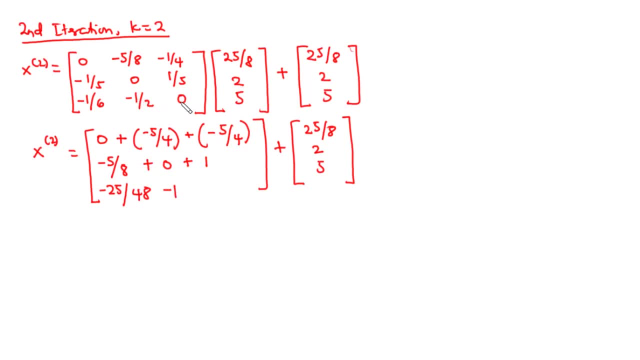 times 2, that is negative, 1.. 0 times 5, that is 0. So we have x of 2 to be equal to considering this matrix we are going to have, when you add 0 and then negative 5 over 4, negative 5 over 4,. 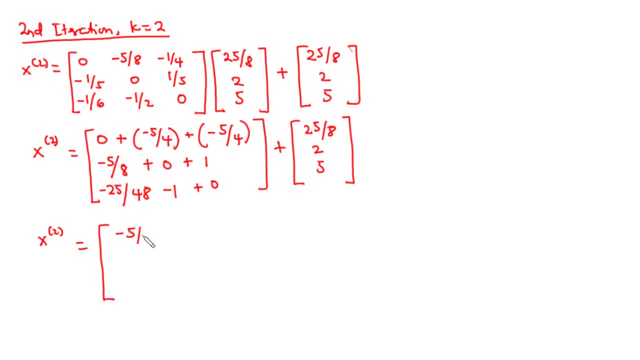 we are going to obtain negative 5 over 2. And then you add this to it: so plus 25 over 8.. And then negative 5 over 8 plus 0 plus 1, that becomes 3 over 8.. And then 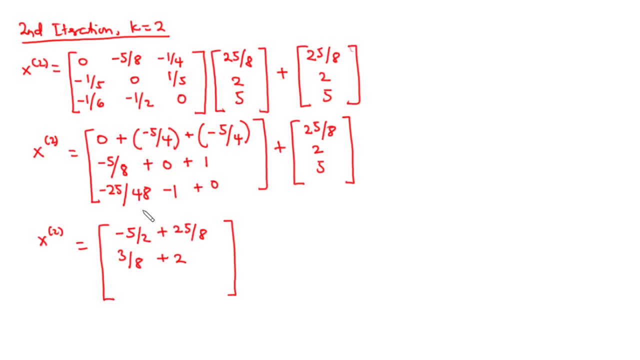 plus 2.. And then negative 25 over 48 minus 1, that becomes negative 73 over 48. And then you add 5 to it, So you are going to obtain 5 over 8,, 19 over 8,.